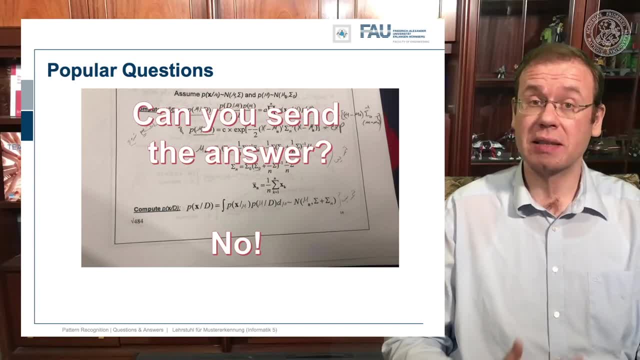 in these videos. I have now the class pattern recognition. I also have the class deep learning and I will answer about the stuff that we discussed in those videos. that's perfectly fine, but I won't solve your exercise problems. yeah, you can save those mails. I won't reply to this, sorry. now let's go. 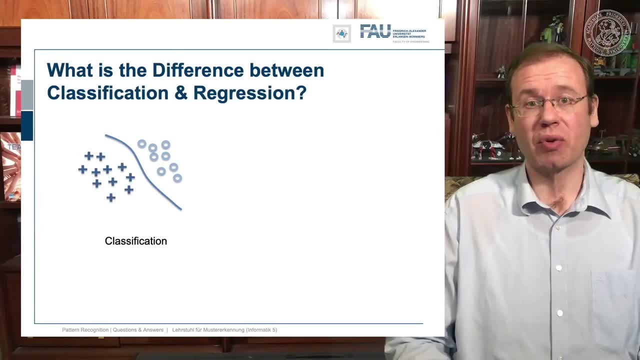 into something where we really had a couple of questions with- and this actually concerns our class- and one question that came up actually in a couple of occasions was: what's the difference actually between classification and regression? now, in classification, as we talked about in the first couple of videos, we want to find the decision boundary and we actually 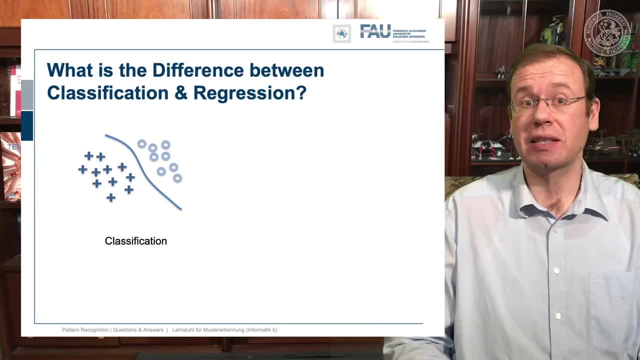 assume that the answer is yes, So we assume that the problem of regression is more or less known to you. so the problem of regression is actually trying to fit a certain mathematical construct. so let's here. this is a kind of curve, maybe a polynomial, maybe it is also a spline, or 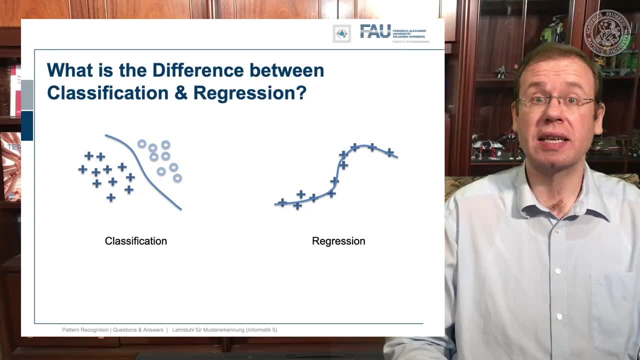 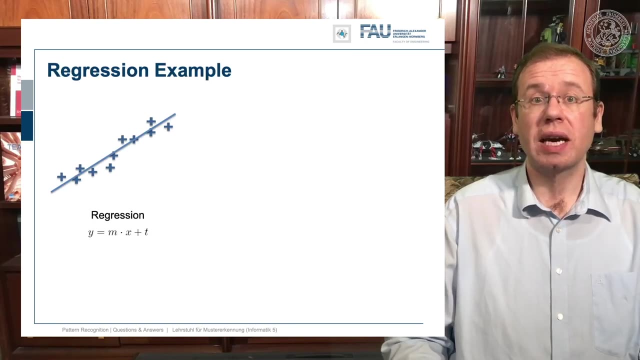 something like this and we try to fit it to the data such that it is able to explain the data and follow it. so this is a regression problem. What you encounter very frequently is linear regression. so in linear regression we have a set of points and we want to fit a line through set of points. Now you 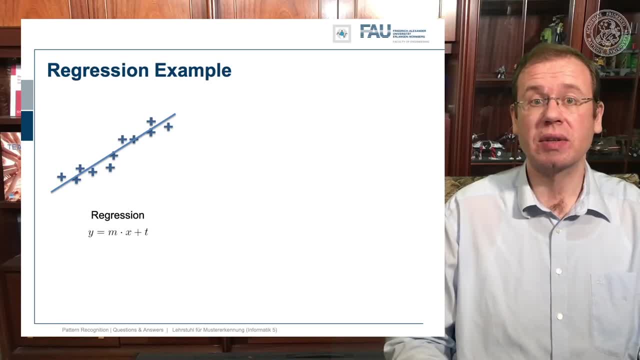 already see that I have a equation here. so this is the kind of model that we try to fit, and we have the observed data x and y and we want to fit the unknown parameters m and t. Of course, to do that I have to tell you what variable is what. 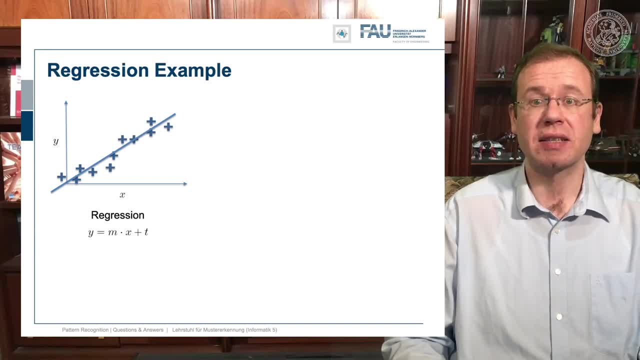 and this is of course the equation here, explained with the axis. So we have the y-axis and the x-axis, And now you can see that with every point I essentially have one observation of a pair of x and y value. Now what we try to. 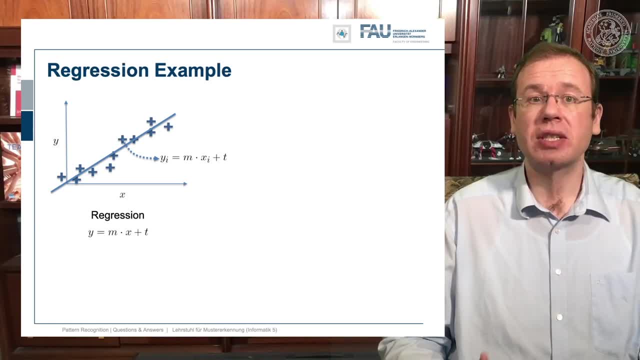 find is the m and the t. that matches this observation best. You see that we have many of those observations. So for every point in the diagram I actually get one equation. So I can rearrange this. Then we end up with a system of equations. You see, I have the y1. that is then. 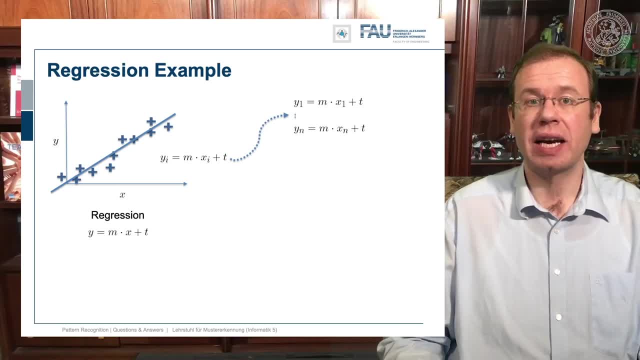 associated to the x1.. And I have the yn, where n is the number of points And this is associated to xn. So we have equations And now that we have many of those equations we can reformat this. And this thing is a system of linear equations. You see here that the y's can be written into. 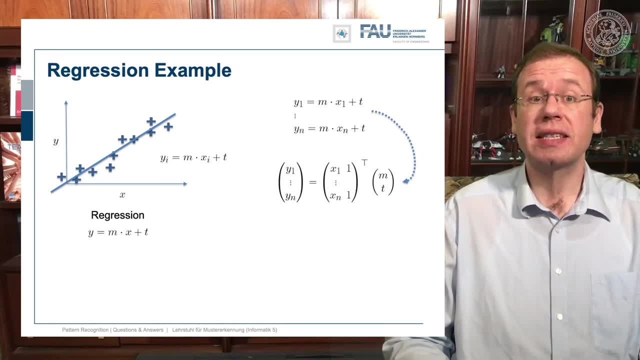 a vector of y, then we can separate the product and the sum on the right hand side and we can express it with means of matrix multiplication. so here, if you take the first line and you do the inner product with the vector mt and you assume in the current line. so let's start with the first line. so this is: 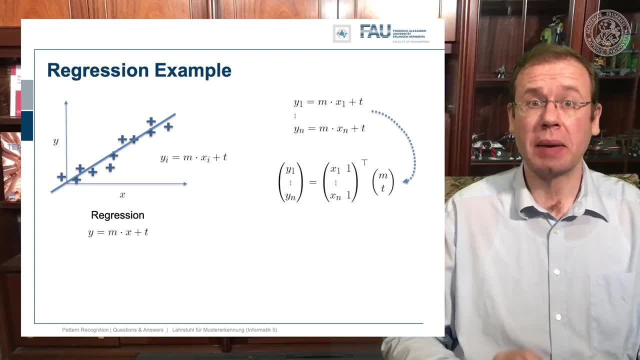 y1 and x1, and now i expand this by essentially a column of ones in this matrix and you see, if i now compute the first line of this inner product, i exactly end up with the first equation. and if i do that for all of the other lines in the system of equations, i exactly get above equations that. 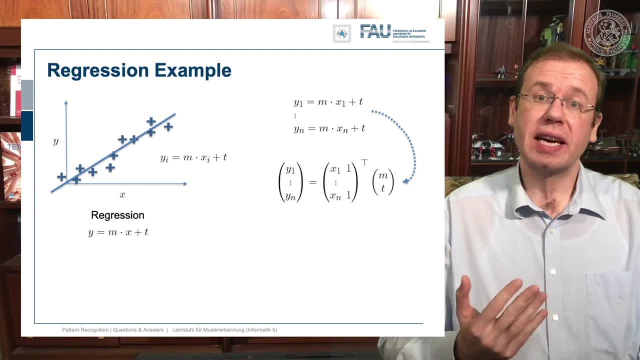 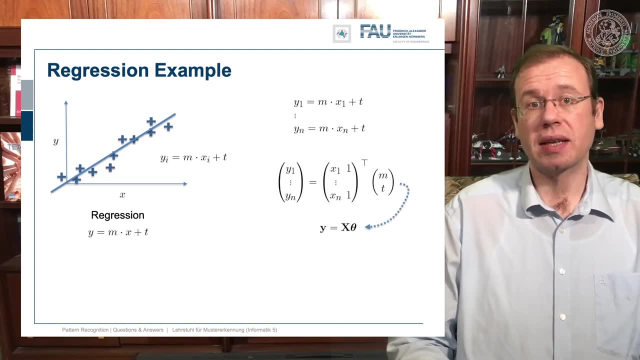 we already observed from the point, so we can rewrite this a little. you can see that the first line of the inner product is the first line of the inner product And you see that this can be expressed completely using matrix calculus. So now we have a vector y, a matrix x and some vector theta. 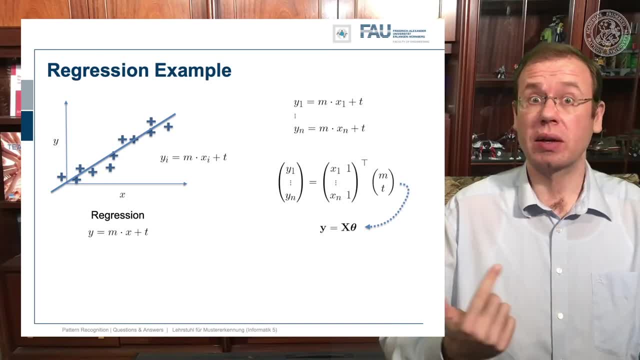 And what you see here is that we can observe all the y, We can observe all the x's, of course also the ones, because they just needed to be associated with the t. So everything is known in x and in y, And all our unknowns are now in the parameter vector theta. 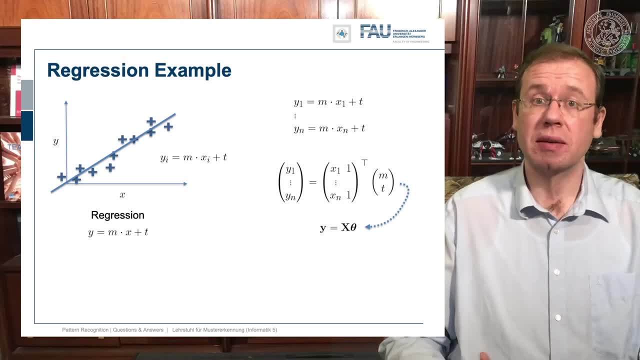 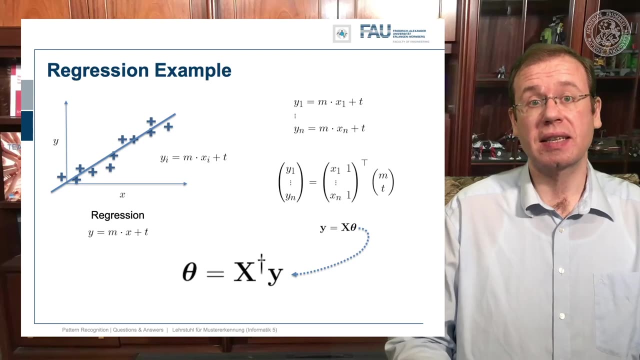 And what we now want to do is we want to solve the system of linear equations with respect to theta, And we do that by computing a pseudo-inverse. So the pseudo-inverse is now multiplied to the vector y, And this gives us an estimate of the parameter vector theta. 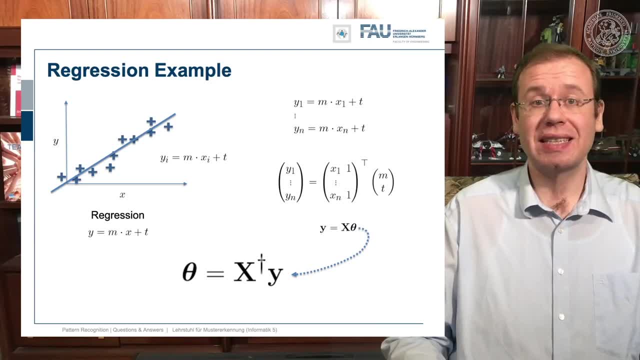 So this would be a least square solution, And this least square solution is typically found then as x transpose x, this matrix inverted and then multiplied with x transpose. So this is the classical pseudo-inverse. So you see, this is a very important concept. 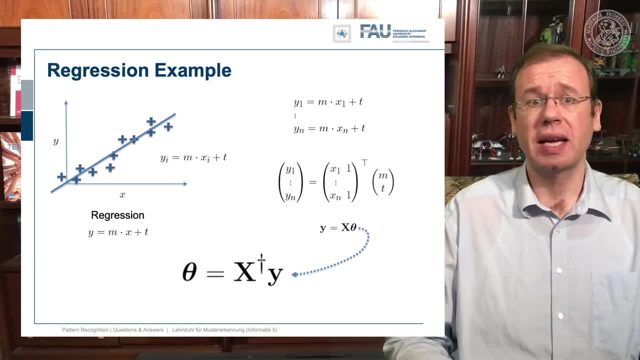 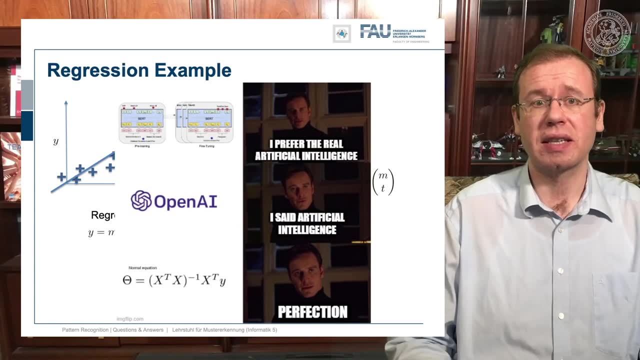 And it occurs all over the place in machine learning And I also found a nice meme for this. So there's all the fancy kind of network architectures and so on, And of course we want to have the real artificial intelligence and there's open AI. 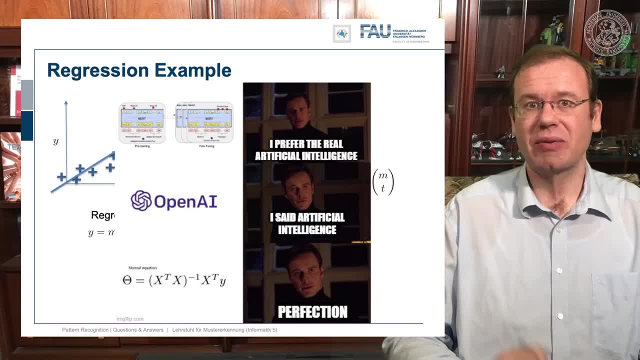 and they also offer a lot of tools, And here we of course want to save artificial intelligence. And then you see, most of the time you then just apply a kind of pseudo-inverse and linear regression And you can solve these things quite easily. 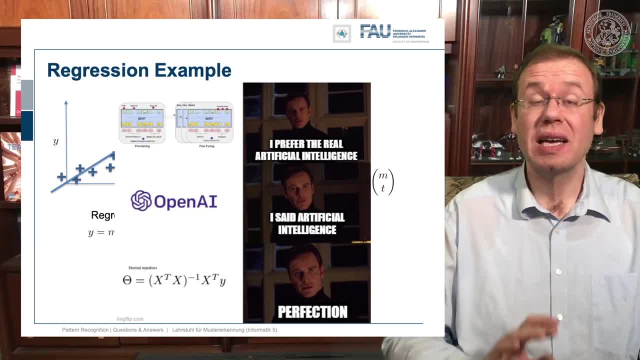 Well, that's not actually the entire thing, But with linear regression you already get pretty far, And if you know how to set up the matrices correctly, then you can even fit polynomials And so on. So linear regression is a very, very nice concept. 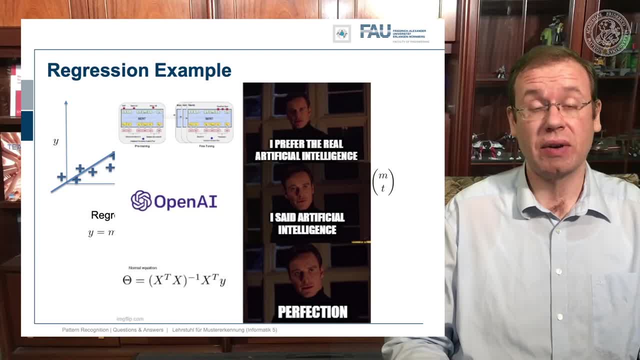 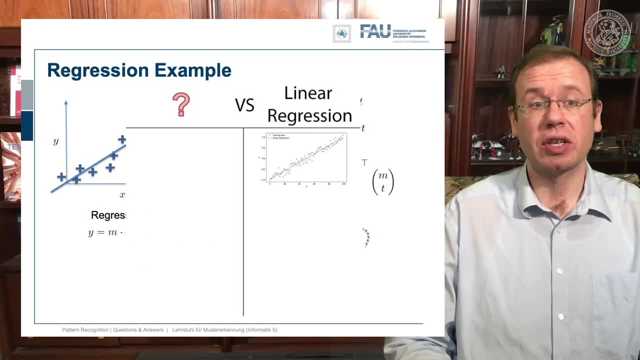 And it's very useful in practical use. It's very frequently employed, So I have a couple of points that are very useful about linear regression. So let's compare it And you see it has explanatory power, It produces a best fit. It only needs a data set. 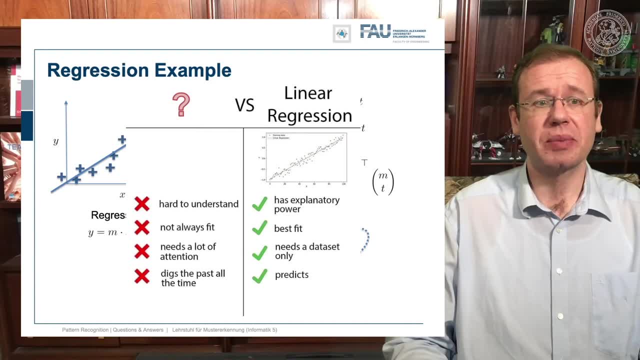 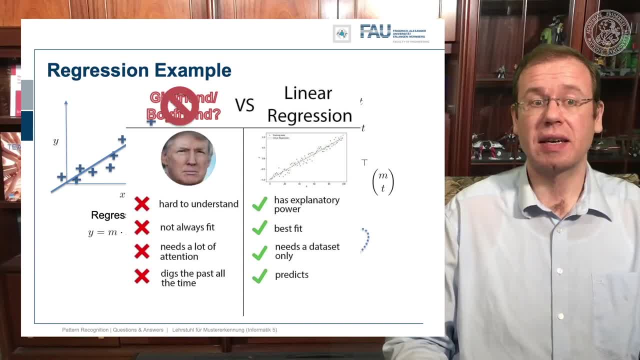 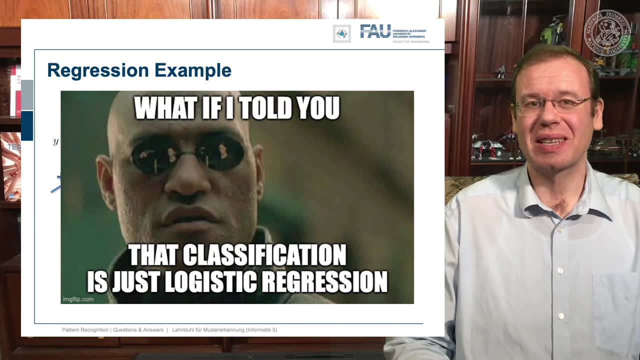 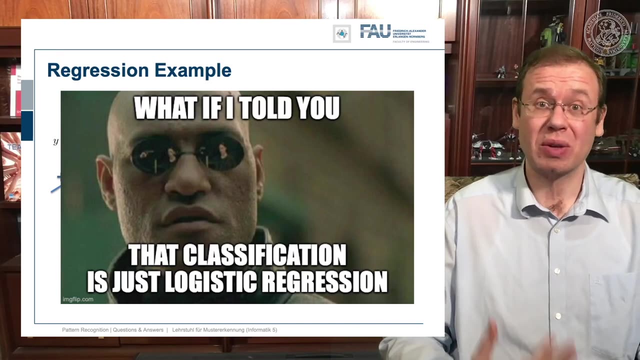 girlfriend. Well, no, It's actually this guy here. So what we've also seen in the lecture, and if you look at the respective episode, you can see then that even the concept of classification can be expressed in terms of regression, because there we are directly fitting the decision boundary. 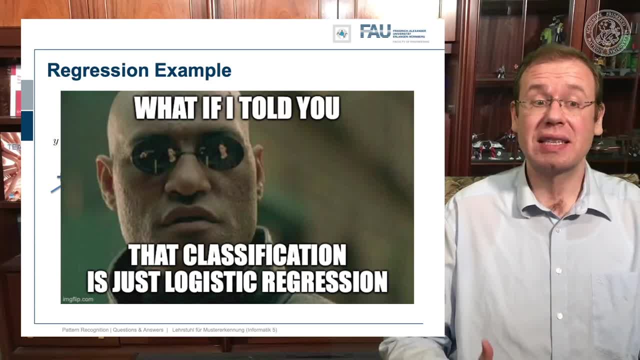 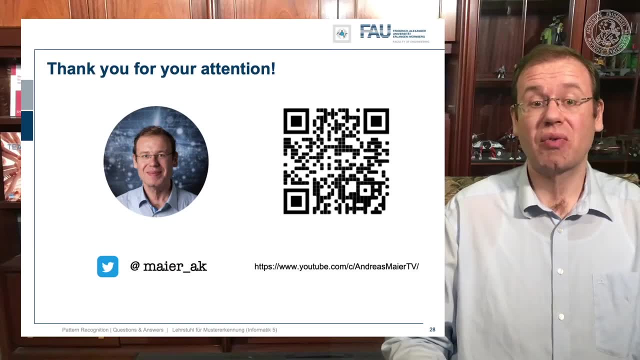 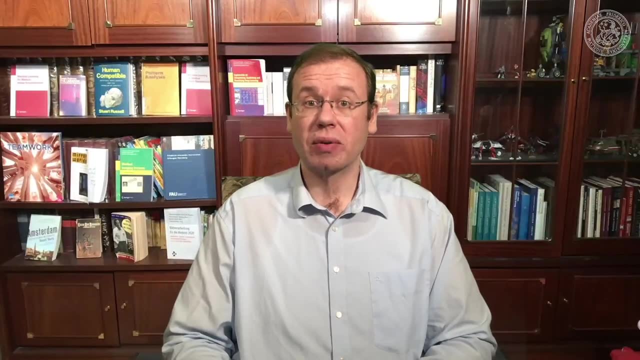 by using the logistic function. So classification. So classification is just logistic regression. So thank you very much for listening And of course I'd be very happy to answer more of your questions. So you can send them, You can leave them as comments.